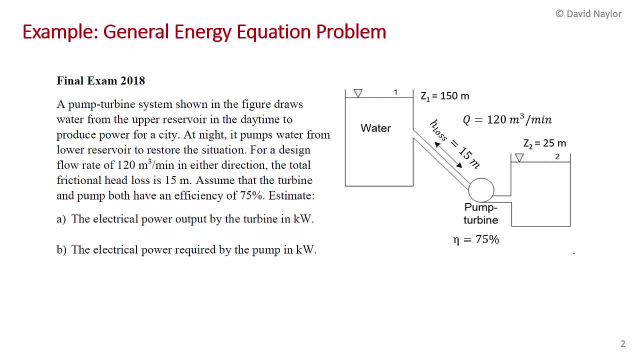 just Doom to viscosity and turbulence is 15 meters, And we're told to assume that the turbine and pump both have an efficiency of 75%. And so in part A we're going to estimate the electrical power output of the turbine during the day when it's providing power. 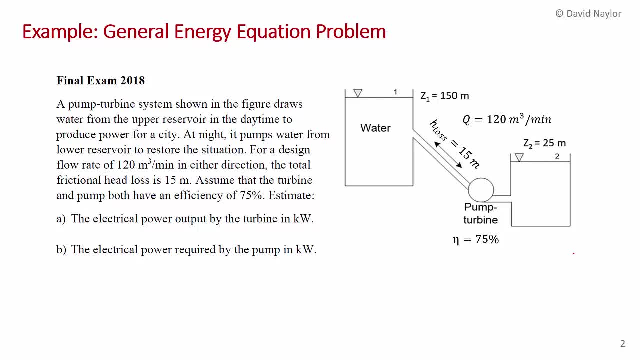 Waters flowing from the upper reservoir to the lower reservoir, And then at part B we've got to estimate the electrical power required to pump the water back uphill from the lower reservoir to the upper reservoir. So you've got to recognize that the flow here is going in opposite directions. 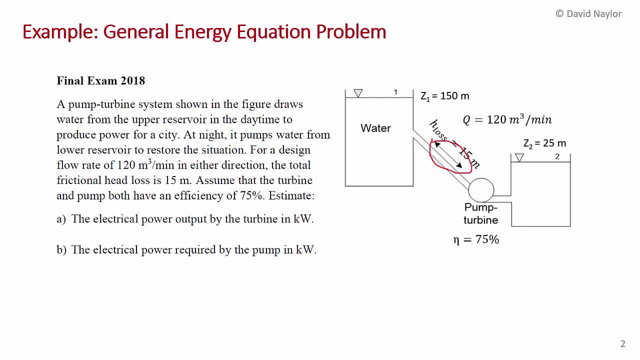 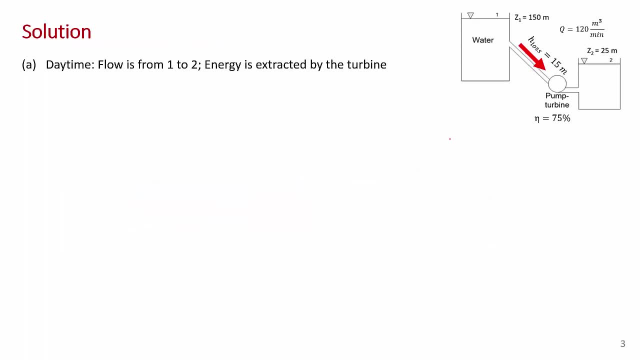 in part A and B, And so you need to write the energy equations in a slightly different form. So here I've shown the problem statement again. This is for the daytime situation. So this is water flowing from the upper reservoir. We're going to call point one is a point on the top. 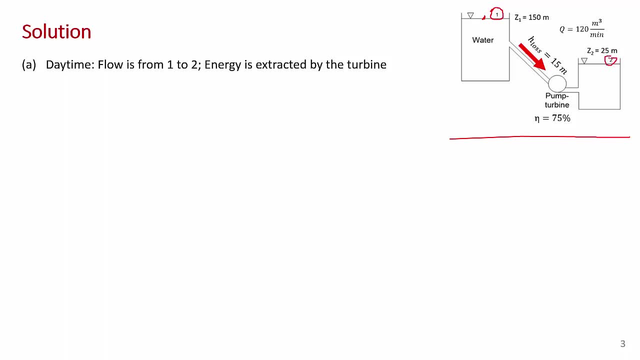 of the upper reservoir and point two here has a point at the top of the water in the lower reservoir. And these altitudes here- Z1 and Z2, are the elevations of the top surface of the water relative to some reference line, some datum. So in this case we're extracting energy with water. 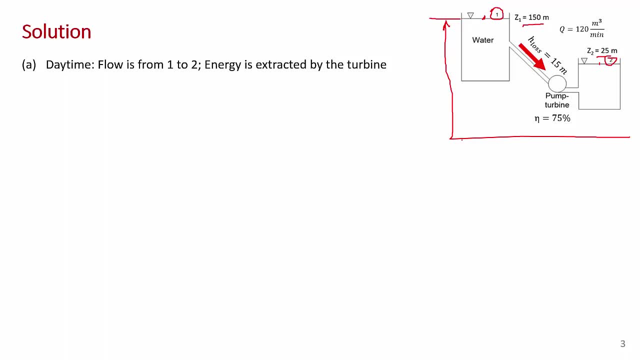 flowing downhill and I've shown that here: A big red arrow with the water flowing downhill and in this case we have a turbine operating with an efficiency of 75 percent. So you start by writing the general energy equation and you want to write the general energy equation with all the terms in energy per unit weight. So 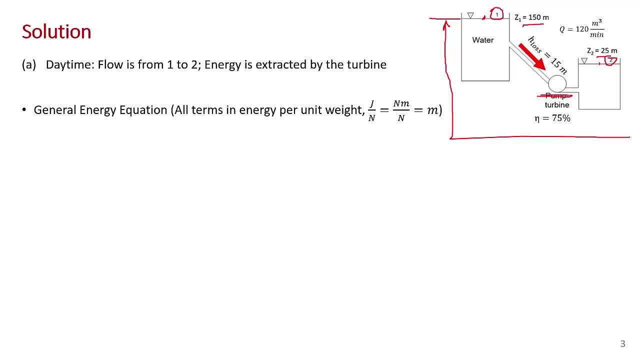 joules per newton or newton meters per newton, and so each term has units of meters, but you want to think of that as energy per unit weight of fluid passing through the pipe. So when we do that, here's the general energy equation written in that form. So P1 upon gamma. 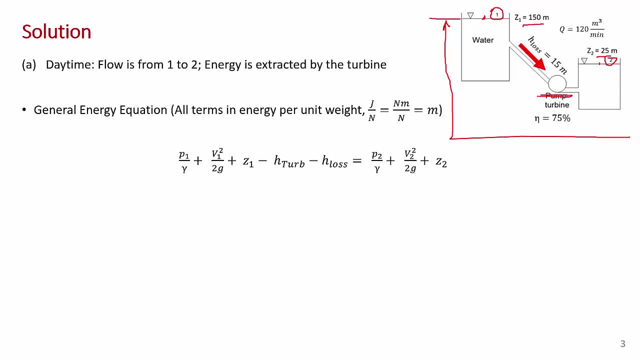 V1 squared upon 2G plus Z1, that's the total energy at point one: pressure, energy, flow, work, kinetic energy and potential energy. So that minus the energy that's extracted by the turbine, minus the energy that's lost due to friction, 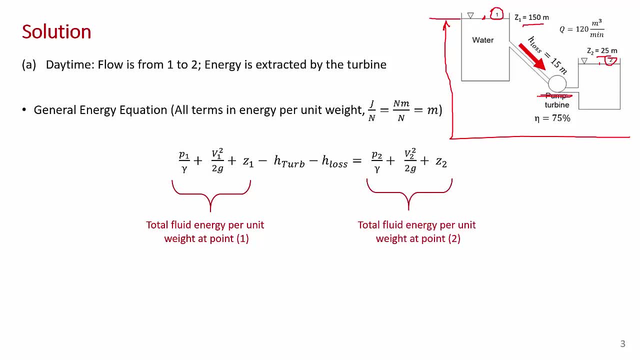 in the pipe equals the energy at two, So P2 upon gamma V2 squared upon 2G plus Z2.. So those are the pressure, kinetic energy and potential energy at point two. This is just simple energy accounting. 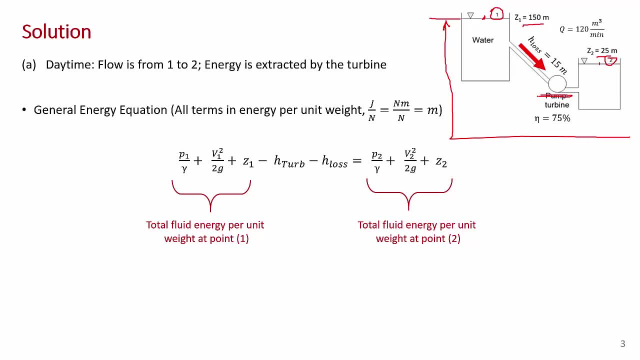 assuming that the flow is going from point one to point two. So we can make a number of simplifications. First off, the pressure at point one and point two. we've assumed these points are right on the surface. here The pressure at the surface is: 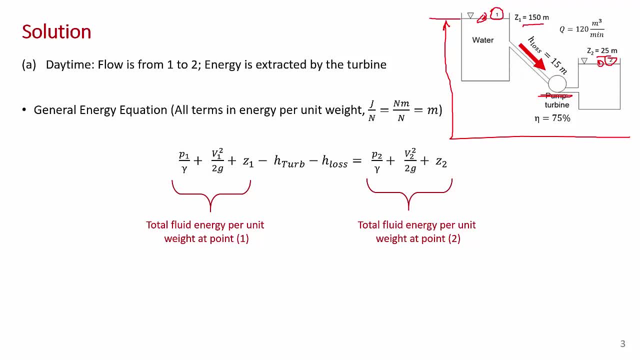 atmospheric pressure. The atmospheric pressure over 125 meters doesn't change significantly, so P1 and P2 are the same. You can either have them as gauge pressures or absolute pressures. In any case, P1 equals P2, so we can cancel those out. Now we've picked. 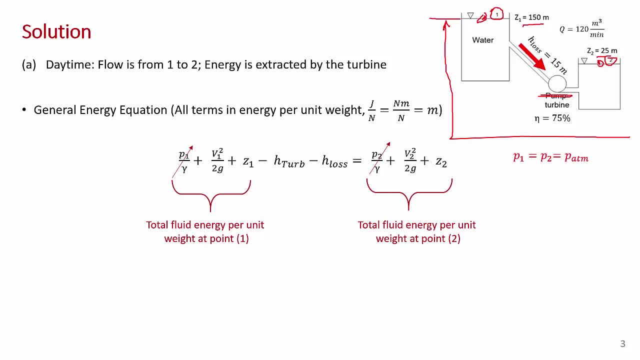 0.1 and 0.2 right at the surface of the reservoir. This is far away from the pipe inlet and the pipe outlet. So at the surface the velocities would be approximately zero. So there'd be almost no kinetic energy. So we can set V1 equal to zero and V2 equal to zero. Now we can solve for the 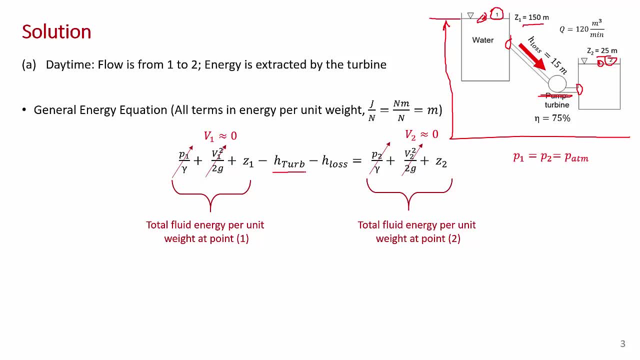 thing we want. We want to find out how much energy is extracted by the turbine per unit of weight of fluid passing to the turbine. That's called the head of the turbine, H-Turb. So we can solve for H-Turb and we get H-Turb equals. you can see Z1 minus Z2, minus the head loss. So you would get 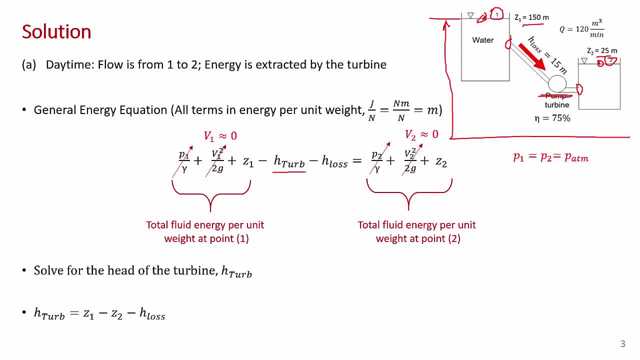 the potential energy of the fluid, That's just Z2.. Z1 minus Z2, but you also lose a little of X energy because of losses in the pipe, And so now we can make the substitutions. The elevation of point 1 is 150.. 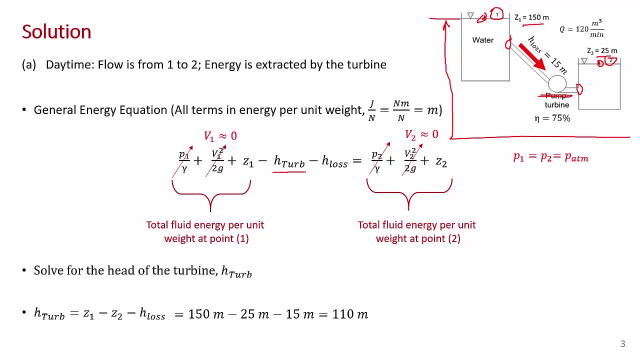 The elevation of point 2 is 25 meters And we're losing 15 meters of head in the pipe. So that's 15 newton meters per newton in the pipe. And so 150 minus 25 minus 15 means that we're extracting 110 meters of head from the fluid as it passes through the turbine. 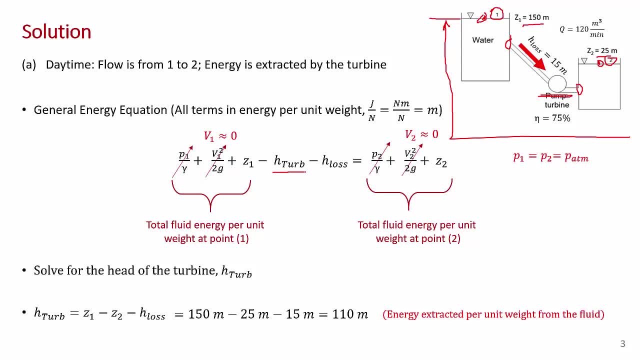 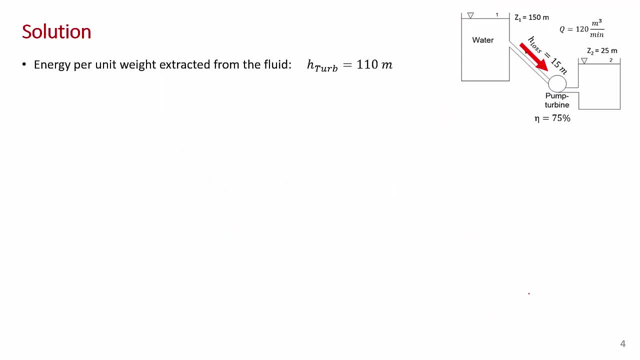 So this is the energy extracted per unit weight from the fluid as it passes through the turbine, And so here I've just written that we've calculated that the energy per unit weight extracted from the fluid by the turbine is a result of 110 meters. 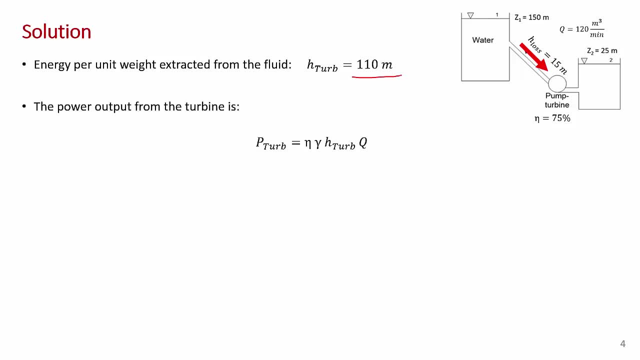 Now, fluid power is gamma, HQ, so the specific weight of the fluid times, the head times, the flow rate. And then we also have for pumps and turbines, we have an efficiency effect here. So the power output from the turbine is efficiency, eta times, gamma of the water flowing through the turbine. 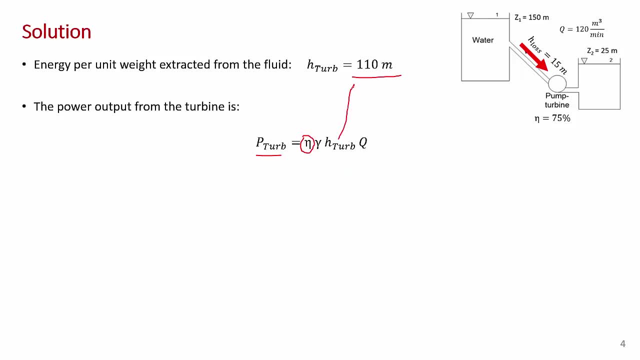 H of the turbine that we just calculated is 110 meters Times the flow rate which you're given in the problem statement is 120 cubic meters per minute. We'll have to convert that to cubic meters per second and we'll do that in a moment. 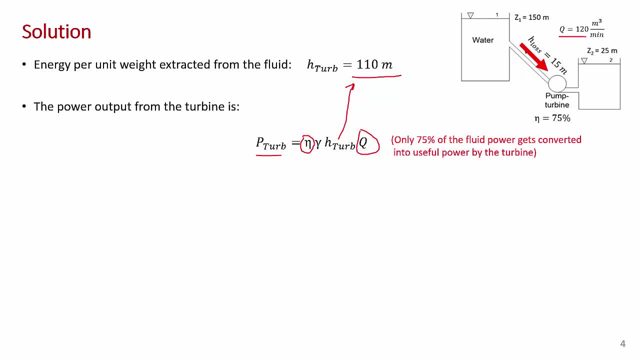 But I just want to point out that we've calculated that the energy extracted from the water flowing through the turbine is 110 meters, In other words 110 newton meters per newton. But not all of that ends up as useful power. 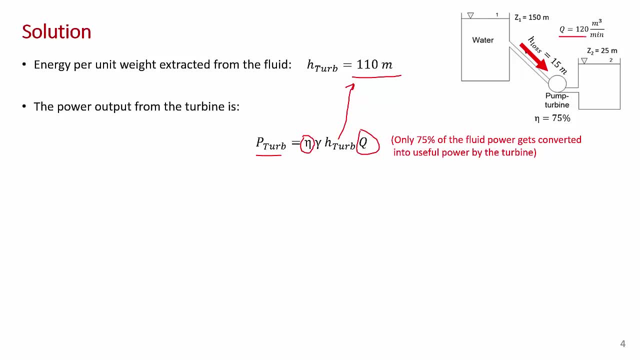 We're going to look at the generator. There's losses in the turbine due to turbulence and well inefficiencies in the conversion of fluid power into shaft power, And so that's why we have this eta effect, this 75% effect here. 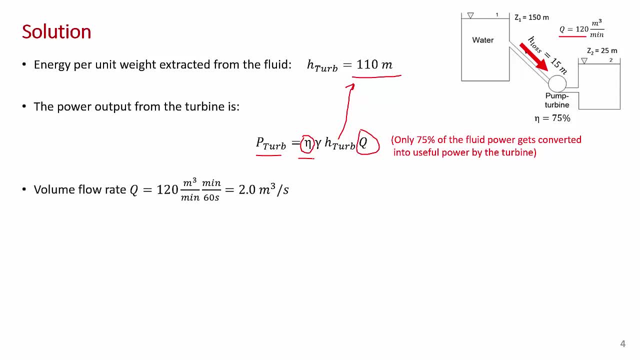 So now it's a pretty straightforward calculation. We need to, of course, convert the volume flow rate from 120 cubic meters per minute, dividing by 60 to get it in cubic meters, So that corresponds to 2 cubic meters per second. 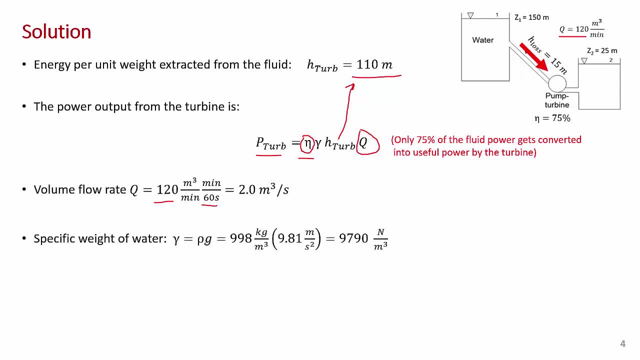 And then I think we have everything to calculate the power of the turbine. Oh yeah, we need to get the gamma of the water, which is the density of the water times g, So 998 times 9.81.. I'm just assuming 20 degrees C water here. 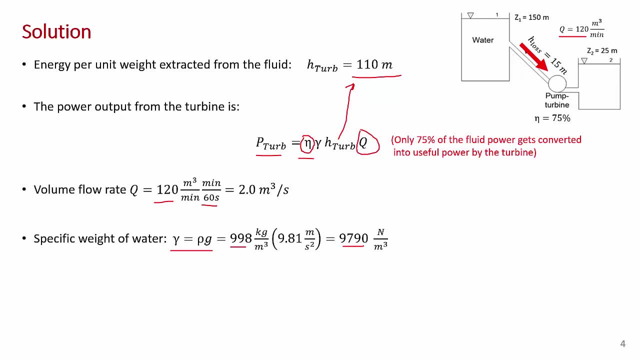 So giving a specific weight of 9790 newtons per cubic meter. Now we can calculate the power of the turbine. So it's eta, Eta, gamma, head of the turbine, times q, So 75.. So 75%, gamma 9790. 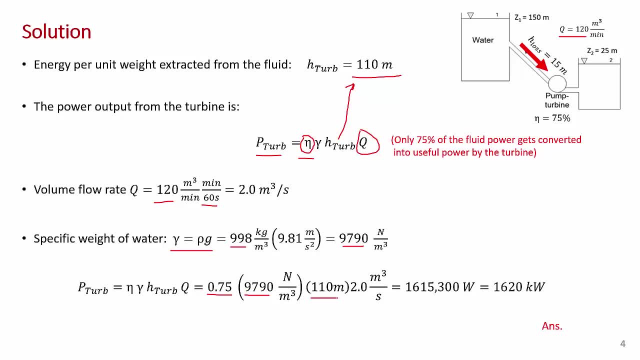 The head of the turbine is 110 meters And then 2 cubic meters per second And you'll see the cubic meters here, go with the cubic meters And you're ending up with newton meter, which is joules per second, And joules per second is watts. 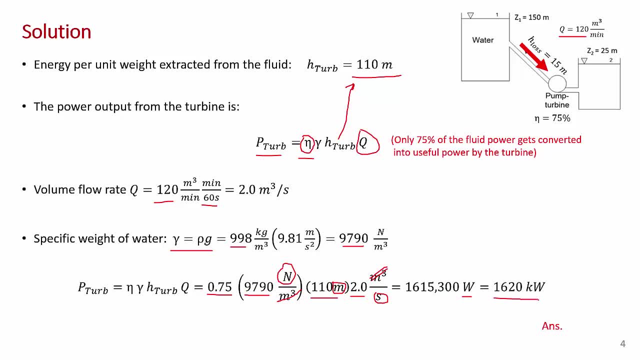 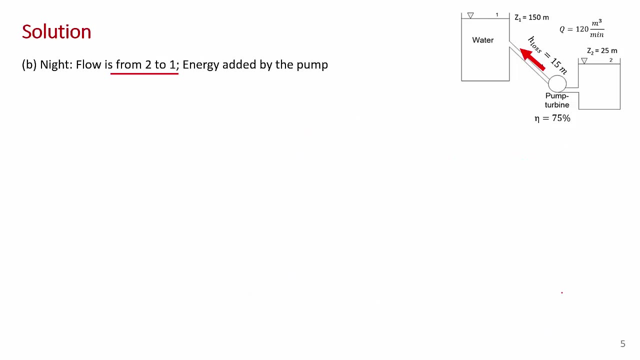 And then I've Converted, divided by 1,000, and rounded it to three digits to get it in kilowatts, So 1,620 kilowatts. And that's the answer to part A For part B. now you've got to realize that the flow is going in the opposite direction. 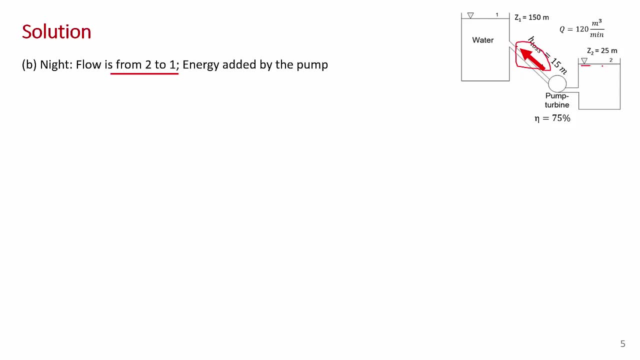 So now we're pumping the water from the lower reservoir to the upper reservoir. This is the nighttime condition when we're trying to restore energy To the upper reservoir. So energy is being added by the pump in this case. So our energy equation. 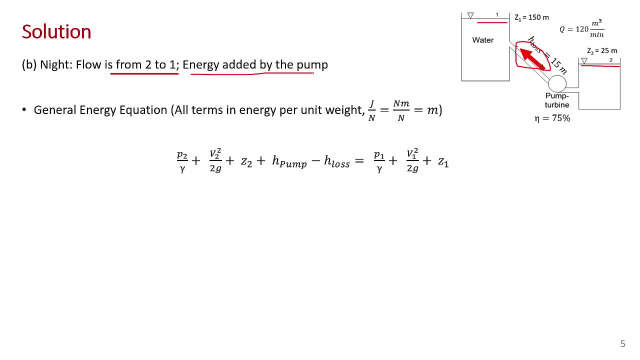 So our general energy equation, again with all the terms in energy per unit weight, is a slightly different form here. Now we're going flow from, We're going from 2 to 1 here Again, considering points right. Point 2 is at the surface of the lower reservoir. 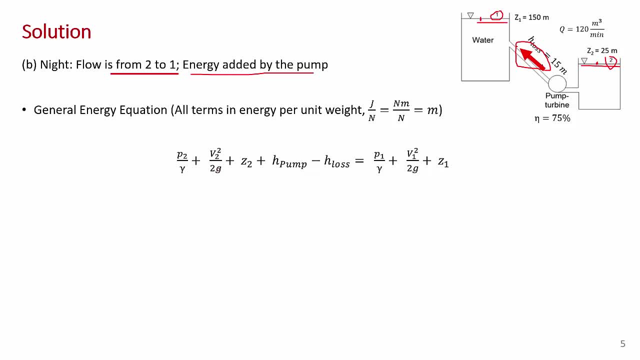 And point 1 is at the surface of the upper reservoir. So now we have the energy at point 2.. Pressure energy, kinetic energy, plus elevation energy, gravitational potential energy. So the energy at point 2, plus the energy to add to the pump, minus the energy that's lost in the pipe, equals the total fluid energy at point 1.. 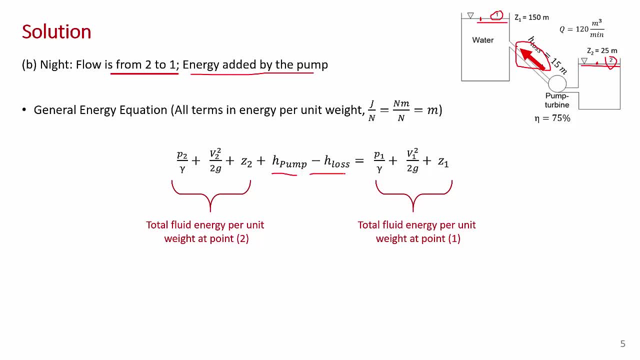 Again we can make the same sort of simplifications: The pressure at point 1 and point 2.. Here is atmospheric pressure which we assume doesn't change significantly over 125 meters. So P1 and P2 cancel out. Similarly, point 1 and point 2 are at the surface of the water, well away from the inlets to the pipe. 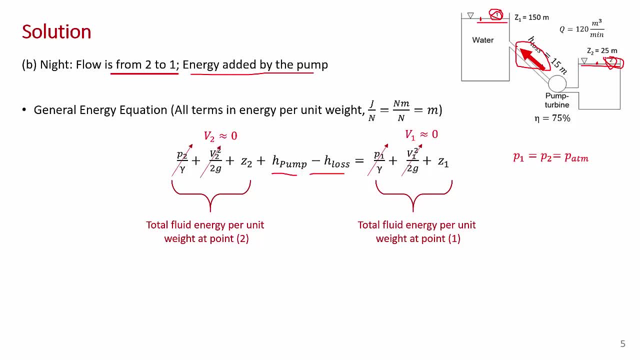 So the velocities at those locations are approximately zero. So now we can solve for the thing that we want: The energy added by the pump. So this is the head of the pump, The energy added per unit weight. Solving for the head of the pump. 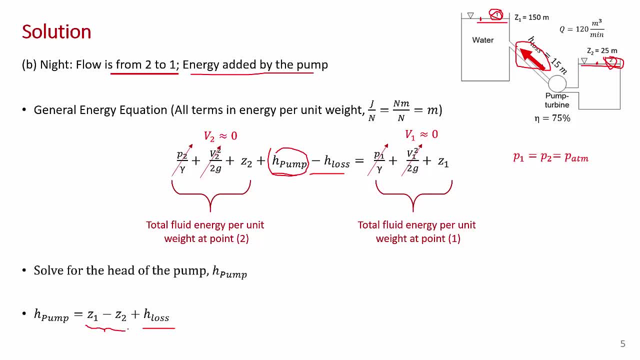 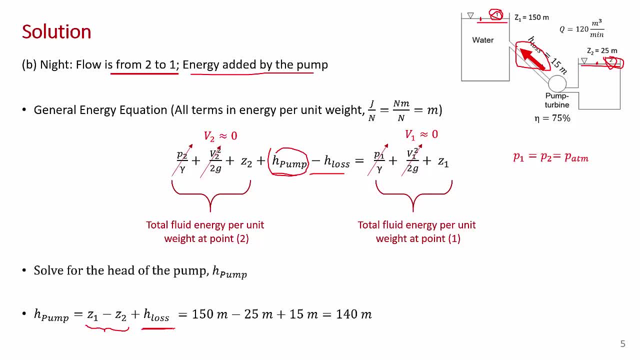 We can make the substitutions. Z1 is 150 meters, Z2 is 25 meters And the head loss in the pipe is 50 meters. So that gives the total energy added that has to be added to the fluid by the pump. 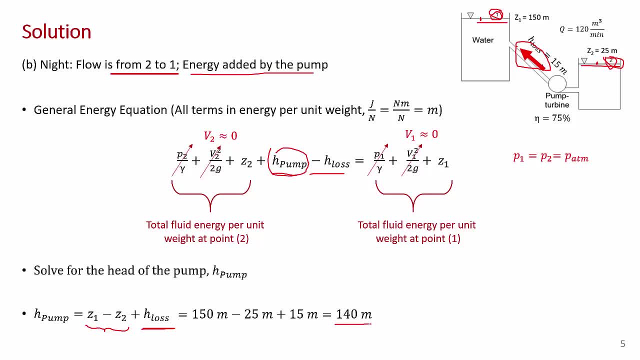 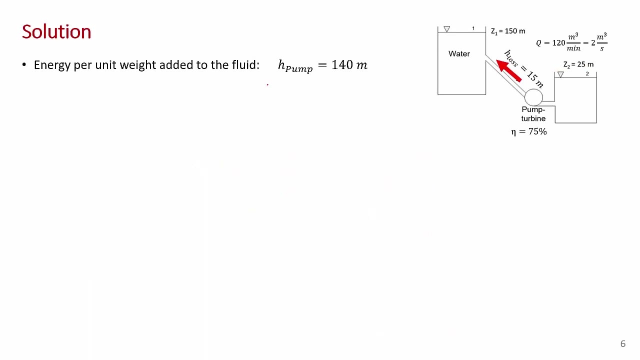 This is equal to 140 Newton meters. per Newton or 140 meters, That again that's the energy added per unit weight to the fluid by the pump. So I've rewritten that result here, that the head of the pump that we've just calculated is 140 meters. 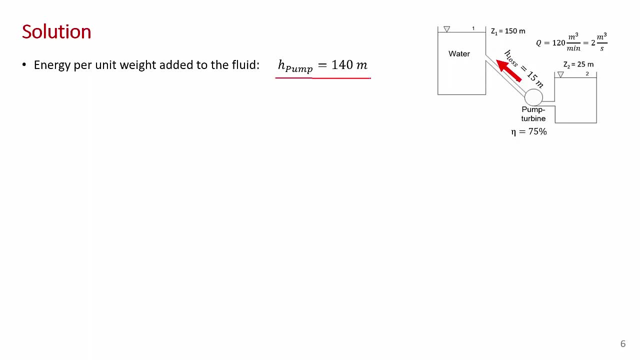 And now we use our definition of fluid power, which is gamma Hq, But it's not a factor. But in this case we divide by the efficiency of the pump. This is because the pump is only 75% efficient in adding power to the fluid. 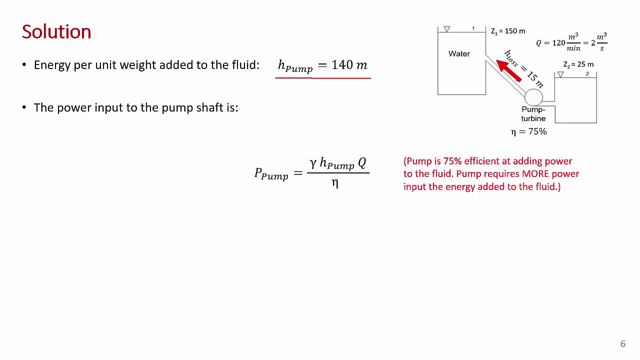 We need to add 140 newton meters per newton and we need to put more energy into the pump because it's not 100% efficient. it's only 75% efficient in transferring energy to the fluid. So the pump requires more power- the shaft power- than is actually added to the fluid. 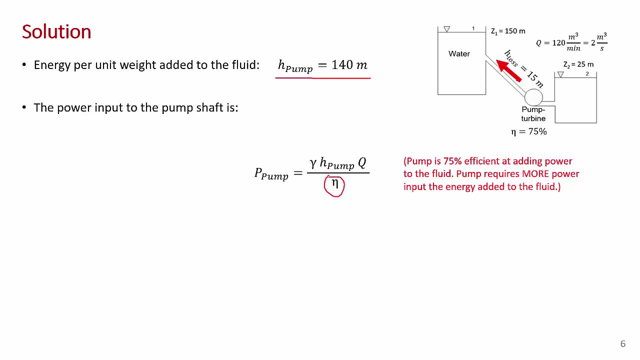 and that's why the efficiency here, eta, is on the bottom. Now we have again. we have that the flow rate is 2 cubic meters per second here. that's basically given in the problem statement and we have the head of the pump here.